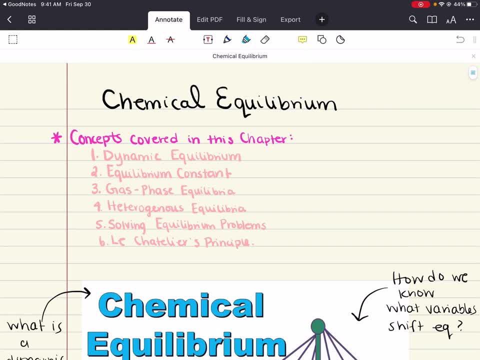 Hello everybody, my name is Iman. Welcome back to my YouTube channel. Today we're going to be talking about chemical equilibrium. The six big topics that we're going to cover here are dynamic equilibrium, equilibrium constants, gas phase and heterogeneous equilibria. We're going to learn. 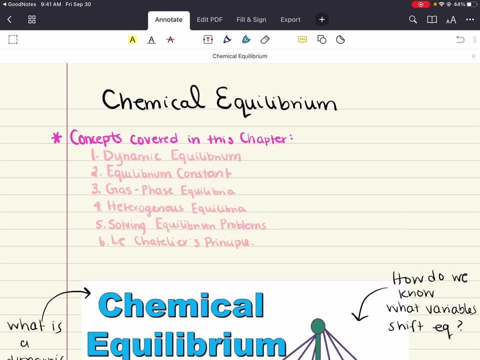 how to solve equilibrium problems and end this chapter with a discussion on Lee-Châtelier's principle. Now in this chapter, we're going to explore the equilibrium that exists between reactants and products in reversible reactions, And we're going to see that a system in equilibrium 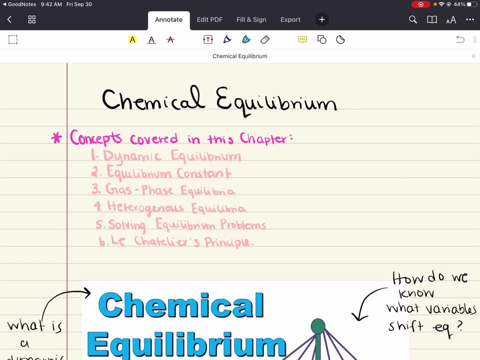 can be described using an equilibrium constant. We're going to learn how to determine the direction that a reaction must proceed in order to reach equilibrium, And we're going to learn about ice tables and how we can use those to solve equilibrium principles. Finally, we're going to 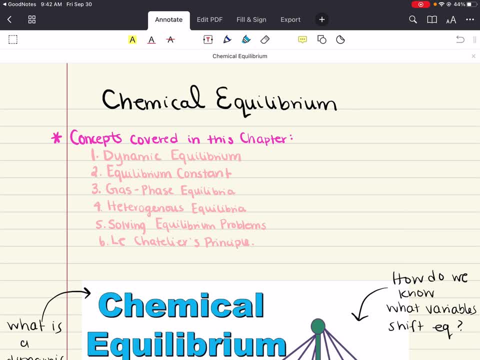 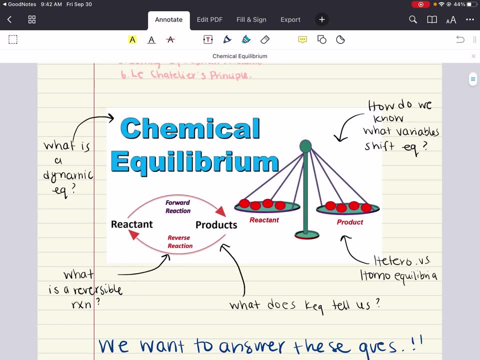 see how a system at equilibrium responds to changes in concentration, pressure and temperature. We're going to answer a lot of really important questions like: what is a dynamic equilibrium? What is a reversible equilibrium? What does KEQ tell us about a reaction? How do 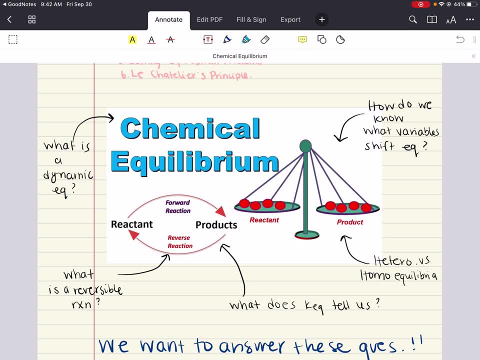 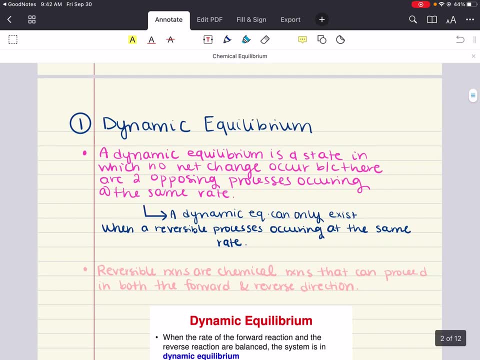 we know what variables shift equilibrium for a particular reaction, And so on and so forth. We're going to answer all these questions and we're going to first start our discussion by talking about dynamic equilibrium. A dynamic equilibrium is a state in which no reaction is possible. A dynamic equilibrium is a state in which no reaction is possible. 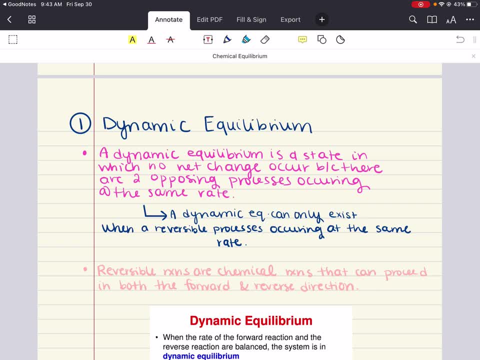 No net change occurs because there are two opposing processes occurring at the same time. Now we've encountered several equilibria involving physical changes, like previously we've talked about vapor. pressure of a liquid Is the pressure exerted by a vapor in equilibrium with its liquid. 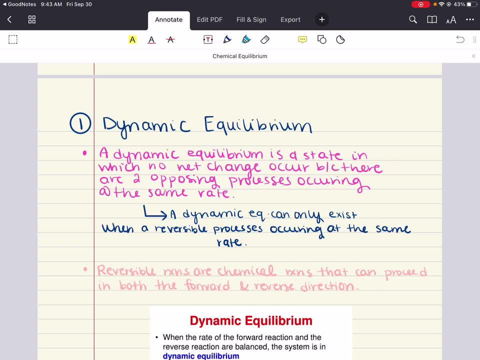 phase And how the equilibrium system is described as a constant change between liquid water and liquid gas. Now, a dynamics equilibrium can only exist when a reversible process occurs in a closed system. Reversible reactions are chemical reactions that can proceed both in the forward and in the reverse directions. When a chemical system reaches 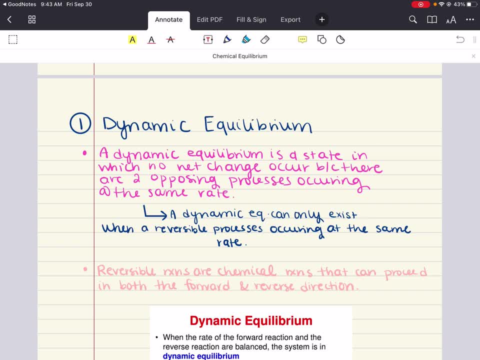 equilibrium. the rate of the forward reaction is going to equal the rate of the forward reaction. the rate of the reverse reactions and the concentration of reactants and products do not change with time. Now, this is a very dynamic process with reactants continuously. 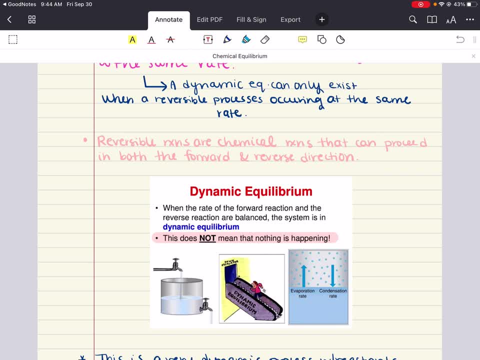 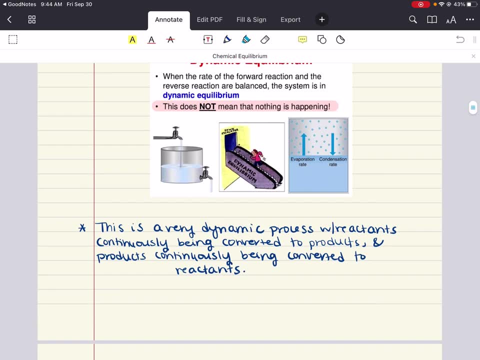 being converted to products and products being continuously converted to reactants. All right, So keep that in mind. When you are in equilibrium, that does not mean that nothing is happening. That is just simply incorrect. Fantastic, All physical and chemical changes tend toward an equilibrium state. Things like to be in equilibrium, in other words. 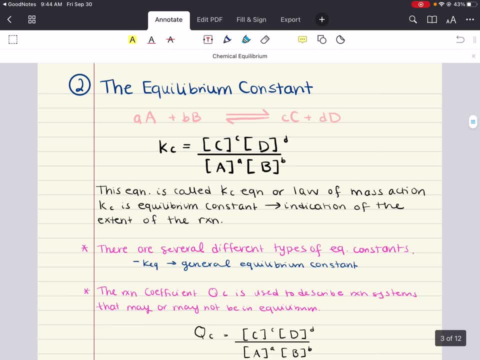 All right. So now that that definition is covered, we can discuss equilibrium constants. Consider the equation that's written here. All right, We have this equation written, All right. We have reactants- capital A and capital B, and we have products- capital C, capital D. 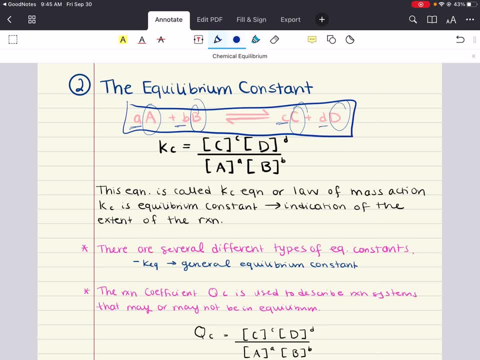 and there are coefficients associated with the reactants and coefficients associated with the products. Now we can write for this equation, we can define the equilibrium constant And this equation is demonstrated here. We're going to put the products at the. we're going to write the products in the numerator over reactants in the denominator. 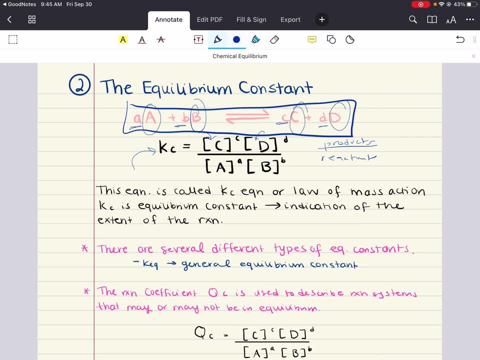 All right, And we write out every product, capital C, capital D, where the exponents associated with that are the related coefficients associated with the products in the reaction. In the denominator we write our reactants: capital A, capital B, Again the exponents that are: 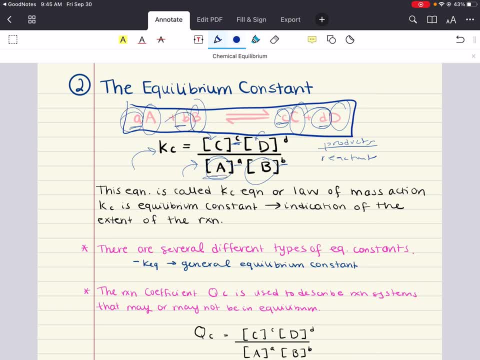 associated with each reactant are the coefficients you see, in the reaction. here This equation is called a KC equation or a law of mass action. KC is an equilibrium constant, All right, And it kind of articulates the concentration, articulates the indication of the extent of the reaction. All right. What that means? 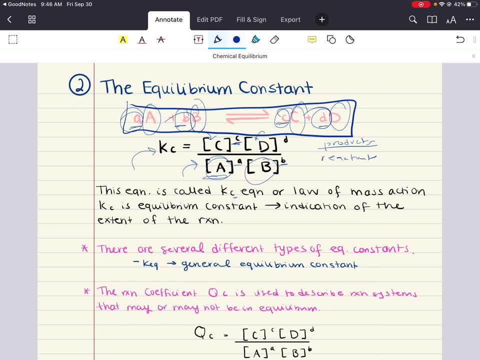 is that the exponents, that the KC equation for any reaction here is going to give us some indication of the extent of the reaction, based off of the value that we can get for this All right? Reaction favors products or reactants as it is trying to reach equilibrium, if it is not already. 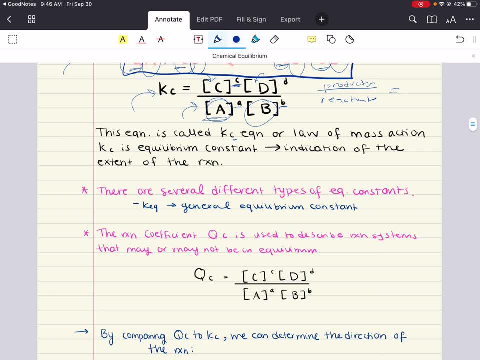 in equilibrium. Now, there are several different types of equilibrium constants. KEQ is an example of a equilibrium constant, and it articulates a general equilibrium constant. In addition to that, you also have your reaction coefficient, KC. This is used to describe reaction systems that may or may not be in equilibrium. Notice it has. 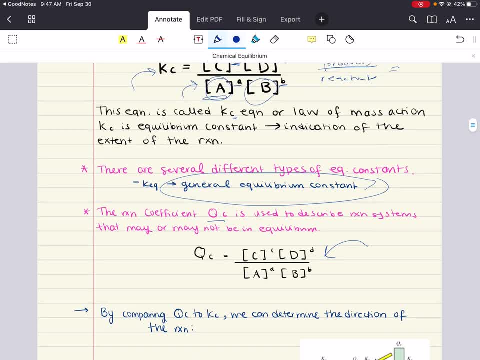 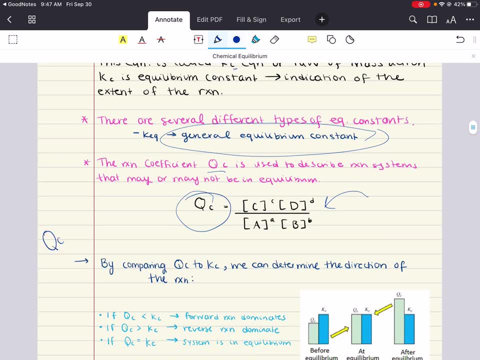 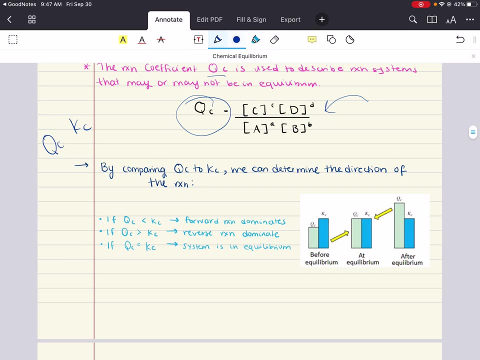 the same format, All right, And it can be used to compare to KC. right, You can compare QC that you calculate for a reaction and KC that you calculate for a reaction, And it can give you some indication, It can give you some information that helps you determine the direction of the. 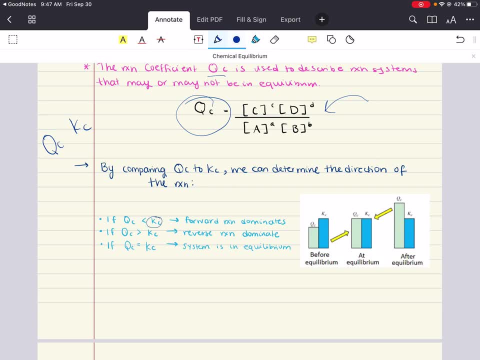 reaction is greater than QC, then the forward reaction dominates. all right, The reaction favors the product. all right, to reach equilibrium. If QC is greater than KC, then the reverse reaction dominates and the reaction favors the reactants. all right, You're forming more reactants to reach. 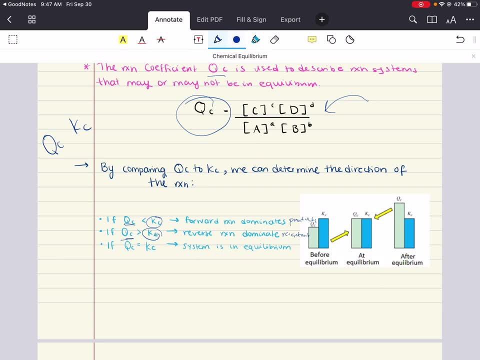 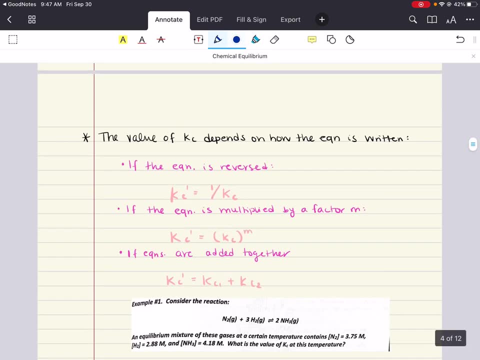 equilibrium, And if KC and QC are equal, then your reaction is already in equilibrium. all right, Now the value of KC depends on how the reaction equation is written. okay, So now, if you have a value for KC and the equation is reversed, all right. the way that you want to write your new KC value is simply. 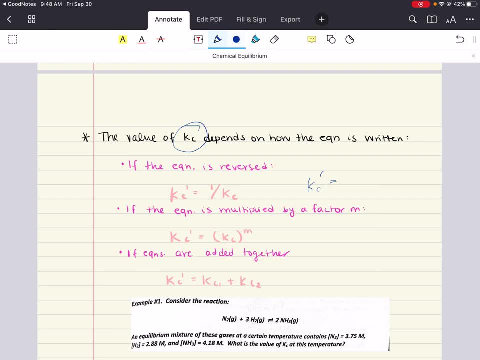 the reciprocal of the original one. So one over your original KC will give you your new KC value for your reversed reaction. If the reaction is multiplied by a factor, then the original KC is going to be raised to a power equal to that factor. all right, So your new KC will be your. 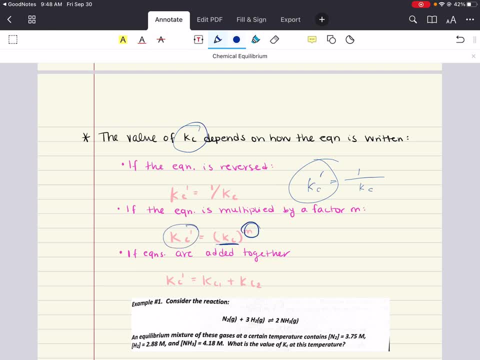 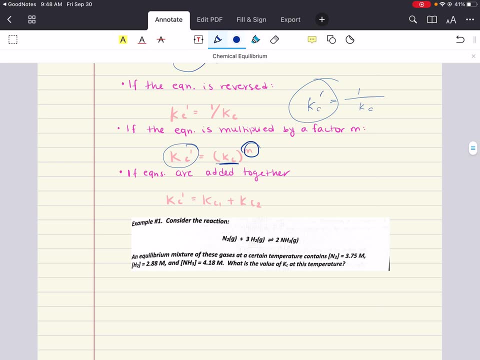 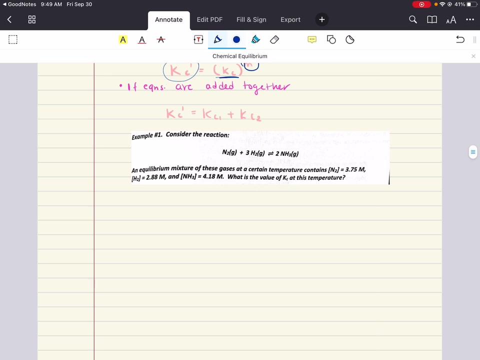 old KC raised to the power equal to that factor. If two equations are added together, the overall equilibrium constant is simply: the product is the addition of two original KC values. Fantastic, This is best understood if we do a few practice problems here. This problem says: consider the reaction An equilibrium mixture of: 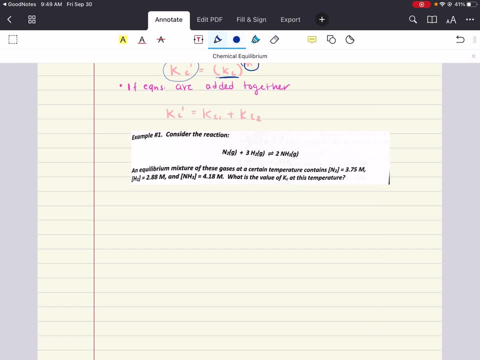 these gases, at a certain temperature, contains Concentration for N2 to be 3.75 molar, H2 2.88 molar and ammonia 4.8 molar. What is the value of KC at this temperature? Let's look at our reaction. All right, here are our reactants, Here are our. 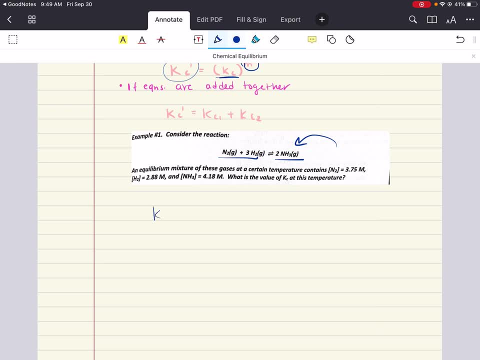 products. This is a balanced equation. So when we're writing the KC for this, all right, we're going to put products at the top. So NH3, all right. this is going to be raised to the power of whatever the coefficient associated with ammonia is, which is 2.. Over reactants we have 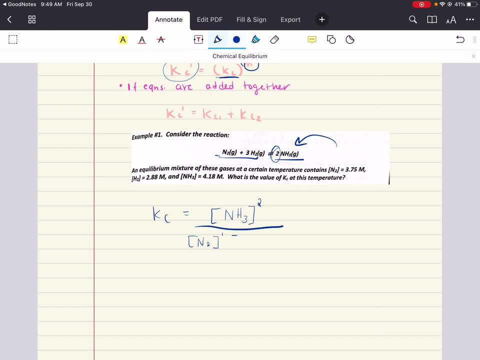 N2.. All right, it has a coefficient of 1.. All right. and then H2, this has a coefficient of 3, so we raise it to the power of 3.. This is our KC expression. Now we can get a value for this by: 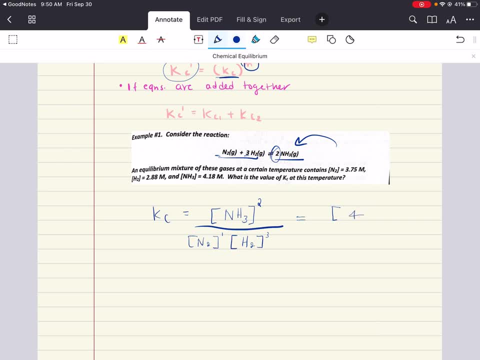 plugging in the values we were given. For NH3, this is 4.18,. all right, molar squared N2 is 3.75 molar to the power of 1.. For H2, this is 2.88 to the power of 3.. We plug this into a calculator. 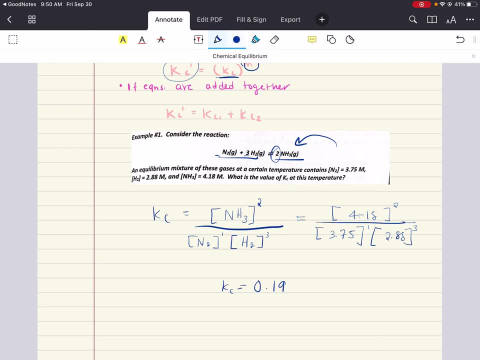 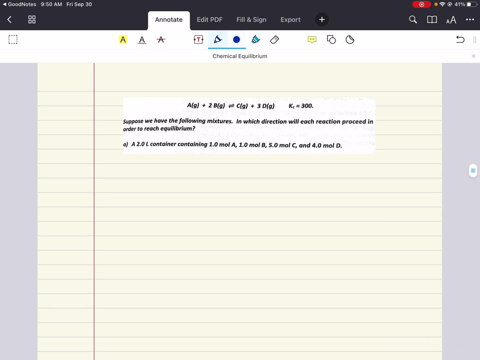 The value for KC that we get is 0.195.. This is the equilibrium constant written without units- Fantastic. Now the second problem says: consider the following reaction: Suppose we have the following mixtures: In which direction will the reaction proceed in order to? 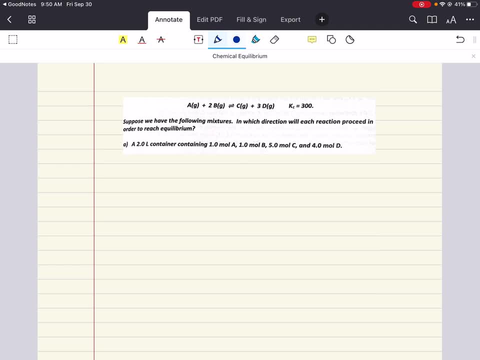 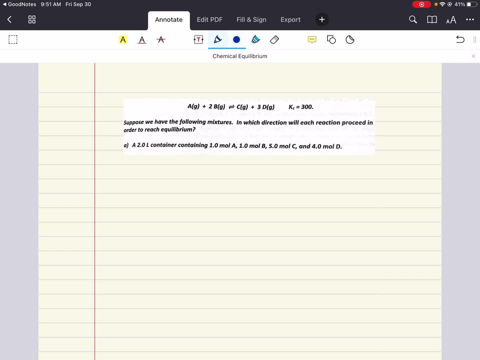 reach equilibrium. All right for this following scenario: we have a 2-liter container containing 1 mole of A, 1 mole of B, 5 mole of C and 4 mole of D. All right, now in order to determine the. 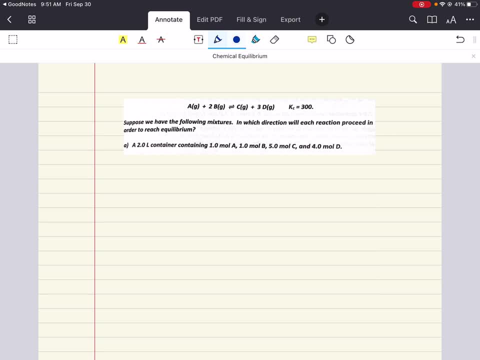 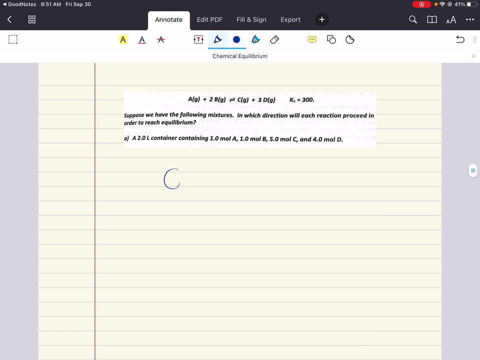 direction of the reaction. we need to calculate the reaction coefficient and then compare it to the reaction coefficient. So we have a 2-liter container containing 1 mole of A, 1 mole of B, and then compare it to our KC value. So first we have to write our QC. all right expression. 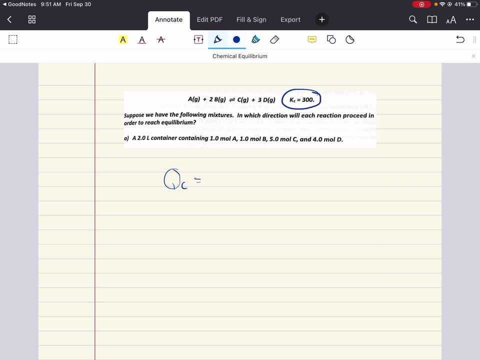 and then we'll compare it to our KC value so that we can determine the direction of the reaction. To figure out our QC we're going to have to write our products on our numerator over our reactants. in our denominator We have product C and product D. Product C: the coefficient. 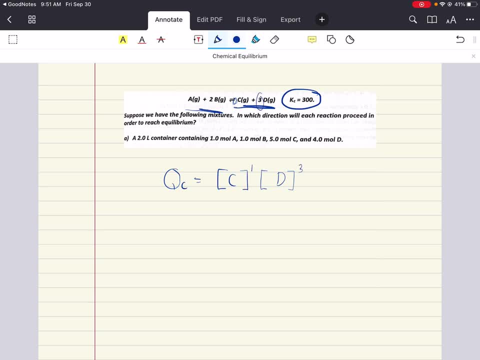 associated with it is 1, and D, We have a coefficient of 3,, so we raise it to a power of 3.. Reactant A has a coefficient of 1.. Reactant B has a coefficient of 2.. Fantastic, All right. so now we have our expression for QC. 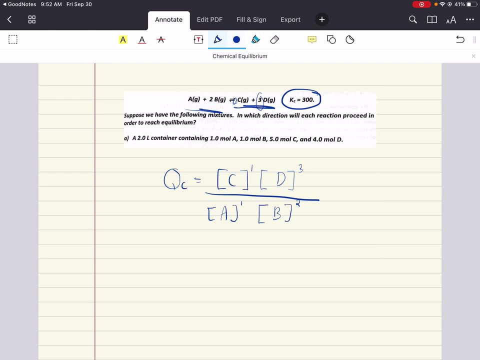 written. Now, when we calculate QC or KC, we have to use concentrations. These concentrations are expressed in molarity, so mole over liters. So we're going to have to figure that out for A, B, C and D, because we're only given the moles. 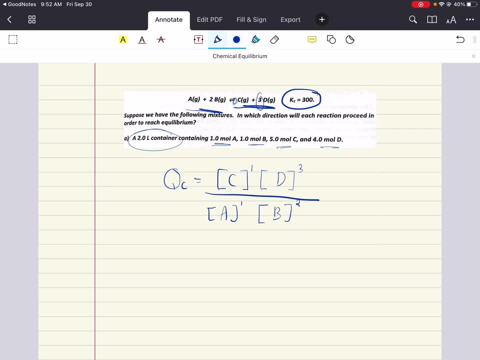 all right. and we know that it's in a 2-liter container, so we have to go ahead and figure out the molarity for each one of these. All right, so for A, we have 1 mole over 2 liters. 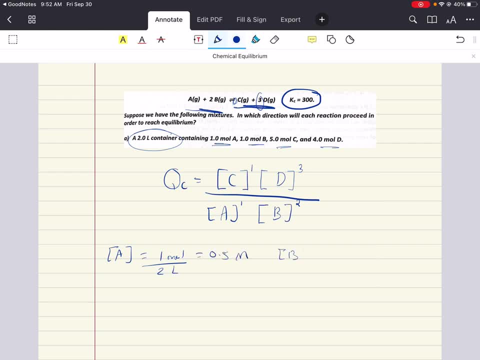 That's going to be 0.5 molar. For B, we are told we also have 1 mole over 2 liters, so this is also going to be 0.5 molar. For C, we have 5 mole. All right, we're going to divide that by the 2 liters we have. This gives: 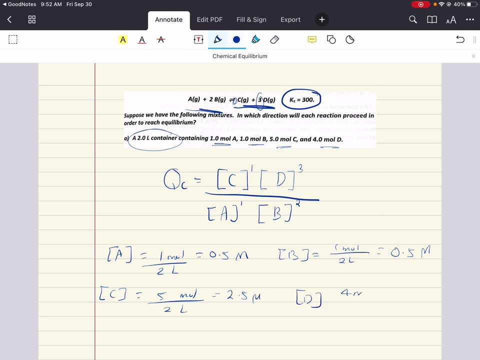 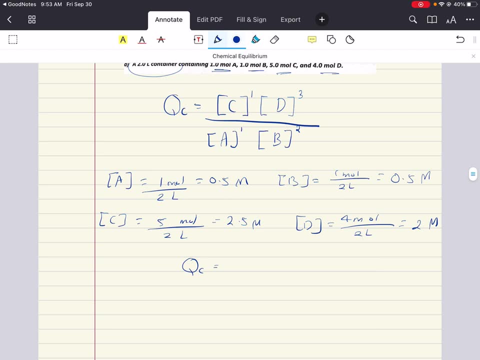 us 2.5 molar, and for D we have 4 moles over the 2 liters we have, and this is 2 molarity. So now when we determine QC, we just plug it in. For C, that's 2.5 to the power of 1.. For D: 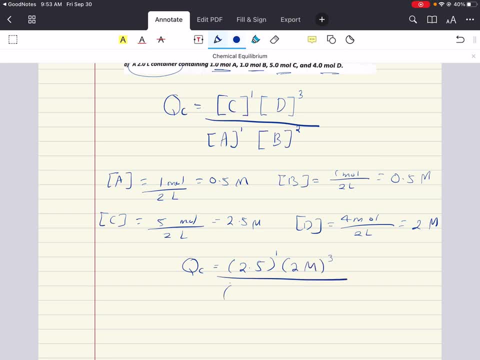 that's 2 molar to the power of 3.. For A in the denominator, that's 0.5 to the power of 1.. For B, that's going to be also 0.5.. If we plug this into a calculator we're going to get 160 for QC. Now we're given the value of 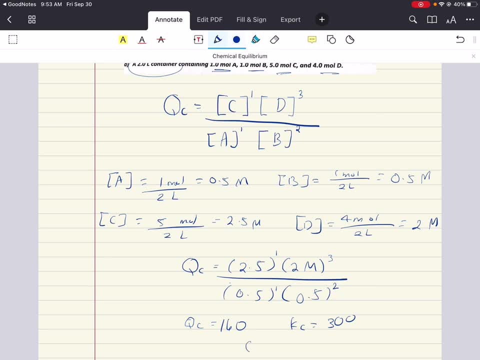 KC, It is 300.. Here, in this case, KC is greater than QC. What does that mean for us? That the reaction will proceed in the forward direction until equilibrium is reached. That means that we're going to form products, more products, more products, more products. So we're going to get. 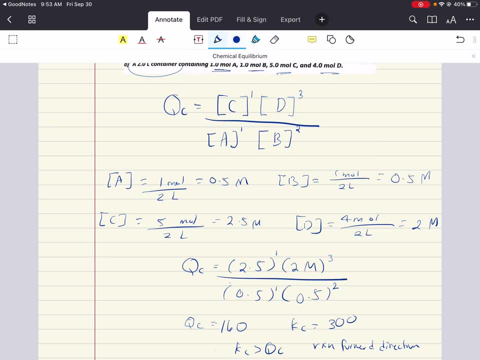 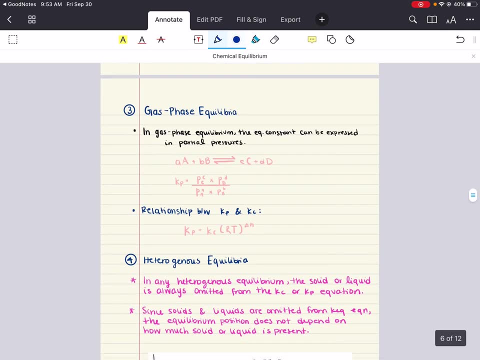 products to reach equilibrium- Fantastic, Awesome. Let's move on to our next discussion. We're going to discuss gas-based equilibria. Here. we're just going to talk about a couple of important points. Same goes for heterogeneous equilibria, and then we're going to jump into. 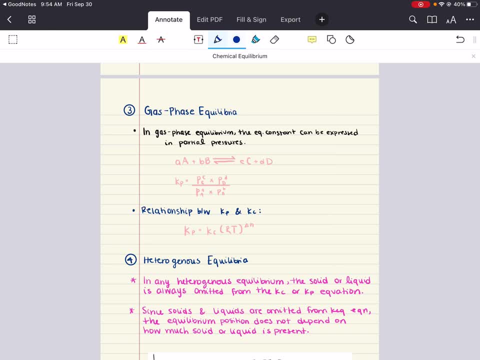 some problems for that. All right. so first is just some definition-based, concept-based discussion. In gas-based equilibria, the equilibrium constant, it can be expressed in terms of partial pressures of each gas in units of ATM or atmospheres. 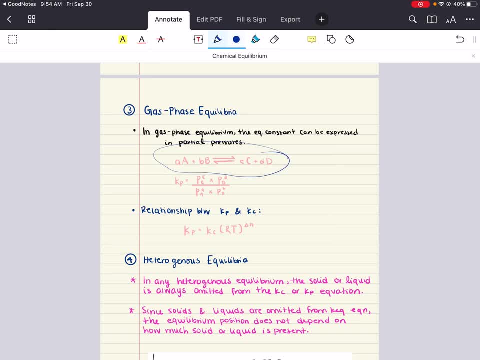 All right. so for this reaction that we see here, all right, for gas-based equilibria, we can actually write our equilibrium constant KP in terms of partial pressures, where we have the partial pressures of our products in the numerator multiplied by each other, raised to. 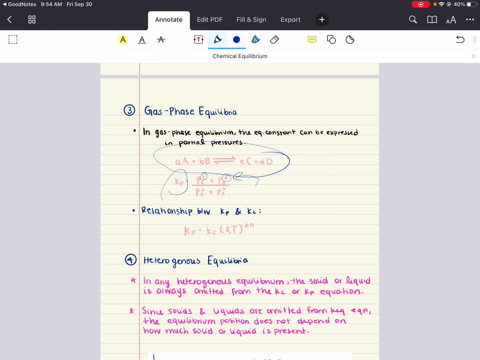 the power of their response. So we can actually write our equilibrium constant, KP in terms of coefficients for the product divided by the reactants in the numerator all right, multiplied by each other for the reactants to the power of their respective coefficients in. 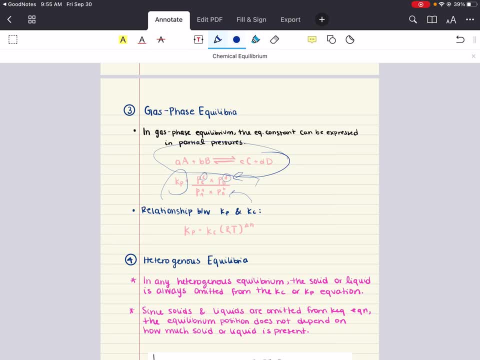 the reaction. Now there is a relationship between KP and KC and it's demonstrated here in this equation KP is related to KC times. the gas constant multiplied by the reactants in the numerator, multiplied by temperature, all raised to the power of delta N. Delta N here represents 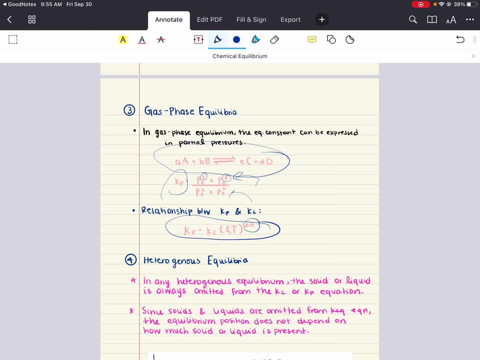 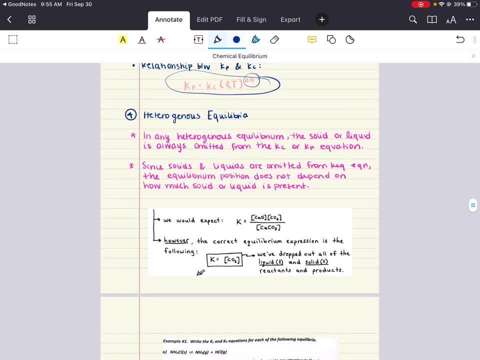 the change in the number of moles of gas in the forward reaction. Fantastic. Now similarly, we can talk about heterogeneous equilibria. In a heterogeneous equilibrium, the solid or liquid is always omitted from the KC or KP equation. We do not write. 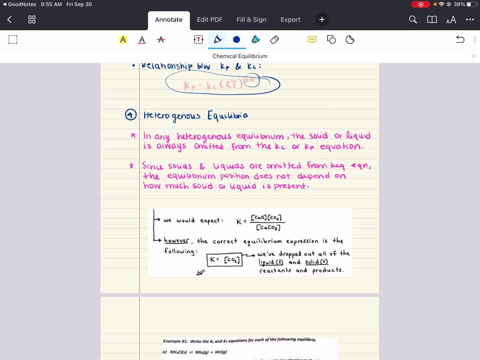 all right reactants or products in our KP and KC equations for any solids or liquids present in the reaction. So since solids and liquids are omitted from equilibrium constant equations, the equilibrium position obviously does not depend on how much solid or liquid is present. 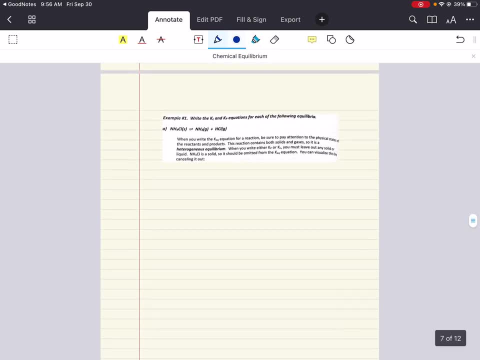 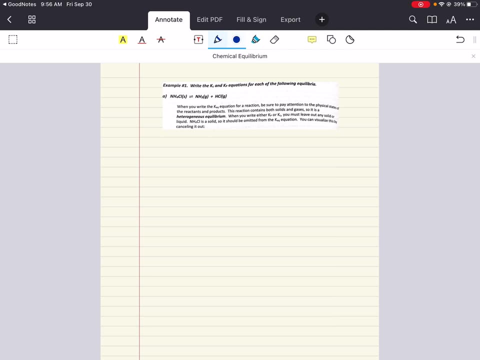 All right. So these are two important things to keep in mind as we move into the next few practice problems. This problem says: write the KC and KP for each of the following equilibria. So we're going to tackle A right here. All right, We have ammonium chloride as our reactant. 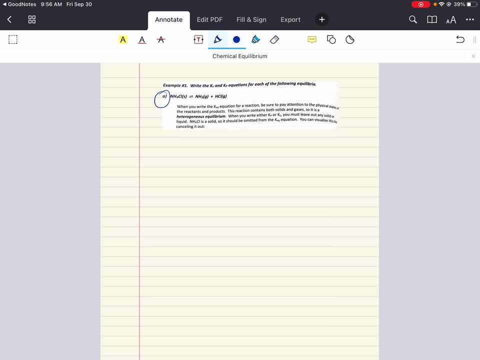 and for our product. we have ammonia and hydrogen chloride. All right, Fantastic. Now there's an important note here: When you write the KEQ equation for a reaction, be sure to pay attention to the physical equation. So if you write the KEQ equation for a reaction, you're going to 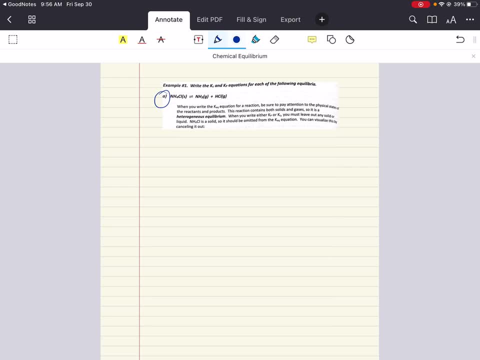 write the physical states of the reactants and products. The reaction contains here, as you notice, both solids- All right, I'm going to highlight that in blue- And it contains gases, All right. So we have a heterogeneous equilibrium here, All right. Now, when you write KP or KC, you have to. 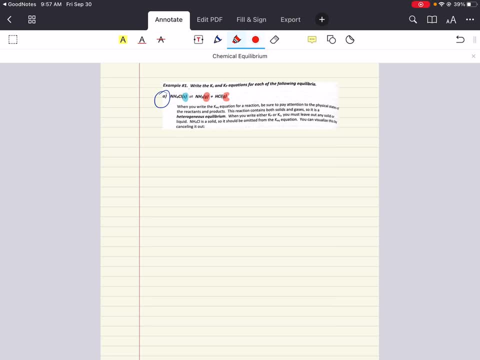 leave out any solid or liquid. So we're obviously going to leave out ammonium chloride, because it is a solid When we write our KC equation. So let's write our KC equation. We're going to write our product, which is ammonia and hydrogen chloride. Their coefficients are both one, So they'll both have. 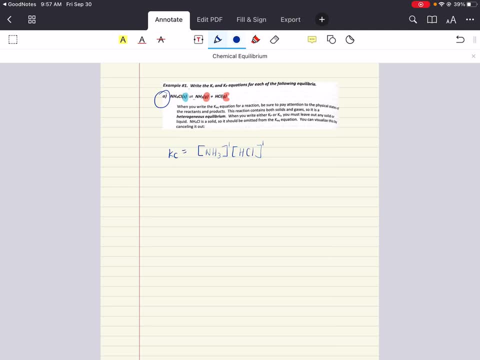 an exponent of one. Now, in our denominator we would write our reactants, But guess what? Our reactant here is a solid, So we actually are going to emit that. In this case, if you're writing KP, you would simply write the pressure of NH3 times the pressure. 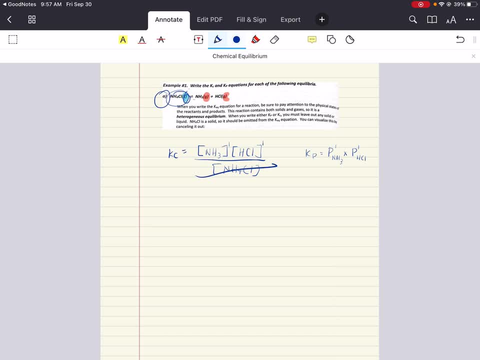 of HCl, because those are our reactants, both to the power of one. Then you'd write the pressure of your reactants, ammonium chloride, but that would be emitted because it is a solid, All right. So then the correct KC equation is just going to be ammonium, All right. And 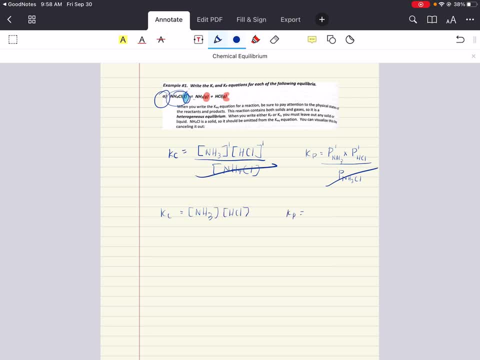 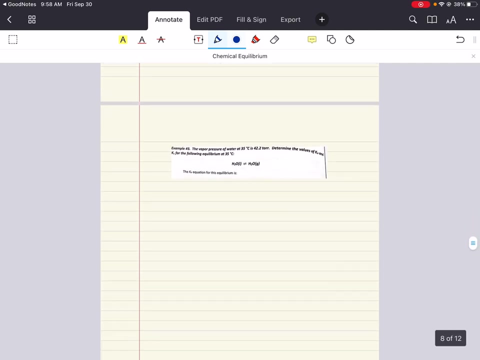 hydrogen chloride And for KP it is simply going to be the pressure of NH3. Times the pressure of hydrogen chloride, And these are our correct KC and KP equations. Fantastic. This next problem says the vapor pressure of water is 35 degrees Celsius. 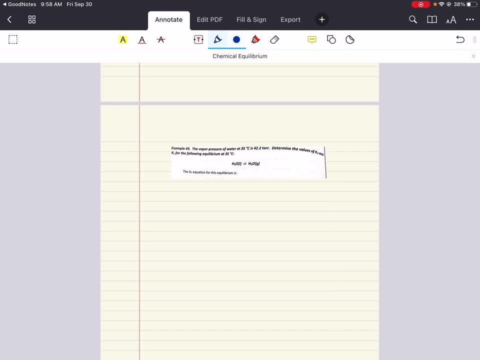 The vapor pressure of water at 35 degrees Celsius is 42.2 torr. Determine the values of KP and KC. for the KC equation, Let's say you have a vapor pressure of 35 degrees Celsius. What you're really trying to do is you're 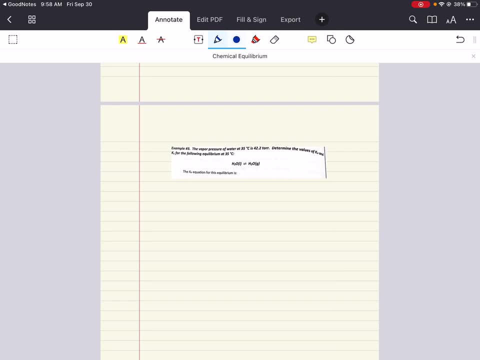 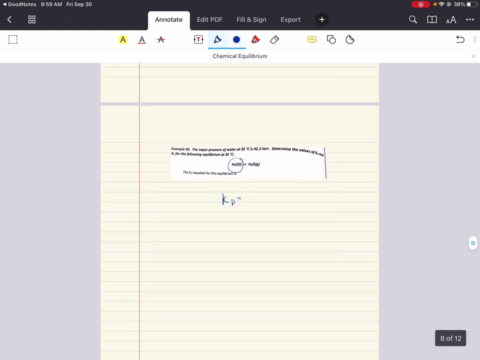 the following equilibria at 35 degrees celsius: fantastic. first thing we want to write is our kp. all right, this is going to be product over reactance. remember: anything that's a solid or liquid is emitted. h2o in our reactants is liquid, so we're going to emit that. what that? 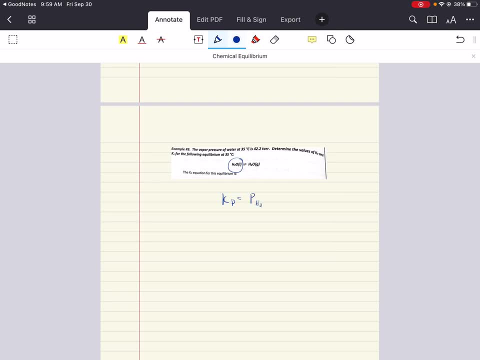 means is: our kp is simply the pressure of h2o and the coefficient of that is one, so it's raised to the power of one. all right, fantastic. so this is the partial pressure of water vapor in units of atmospheres when the system is in equilibrium. so in order to solve this problem, we obviously 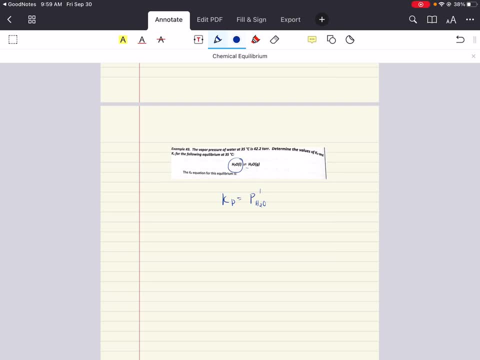 need to know the definition of vapor pressure. okay, we know that vapor pressure from previous chapters is defined as the pressure exerted by a vapor in equilibrium with its solid or liquid phase. so here, since vapor pressure is, as a is by definition, an equilibrium value, it is the same as 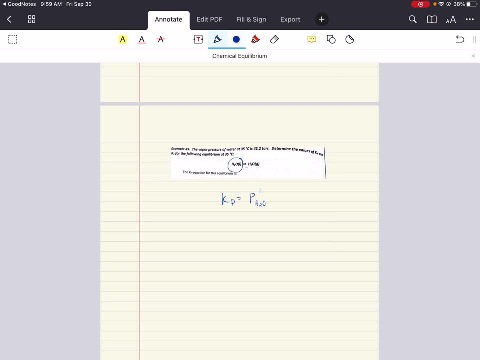 the uh partial pressure of h2o in this kp equation above. the only thing we need to do is convert tor to atm, because kp values are determined- notice: kp values are determined from partial pressures of gases expressed in units of atom atmospheres. so that's a lot of words. um, that's a lot of words to say that this vapor pressure. 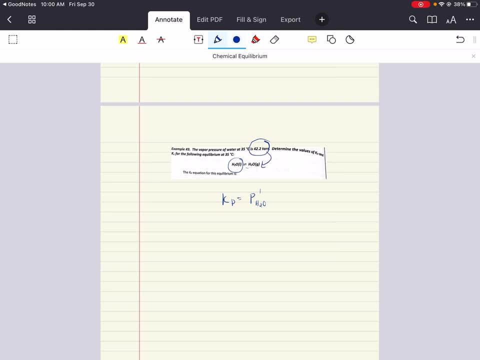 you're given. all right is the vapor pressure here that we are trying to determine in our kp equation. the only thing we need to do is convert it to atmosphere. so we're going to do some dimensional analysis. 4.2 tor is equal to: for every. for 760 tor, that's equal to 1 atmospheres. right, that way. 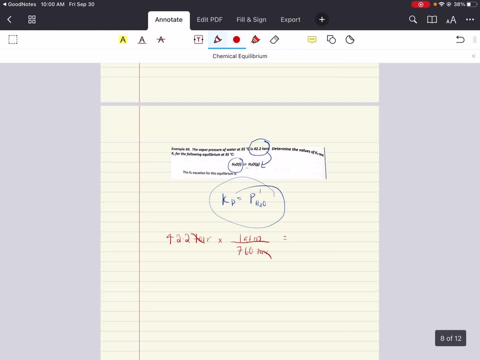 we can cancel the units of tors and have this simply in units of atmosphere. plug this into a calculator. we get 0.055 um, five atmospheres. perfect, now we're gonna use this value for the kp equation. all right, we don't we? we don't write units, though, because kp values are unitless, so 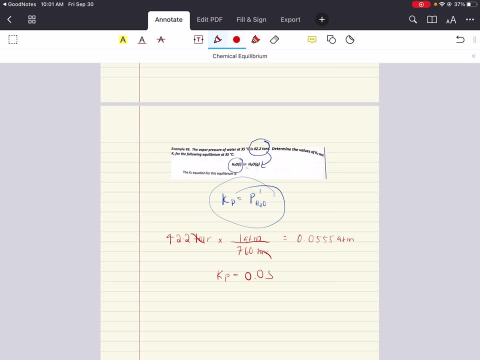 we now know that our kp value is zero point zero, five, five, five. now that we've determined the kp, we can use our relationship equation to determine kc. all right, kp is equal to kc. all right rt to the power of delta n. now we can rewrite this so that we can have a equation for just kc. all we have to do. 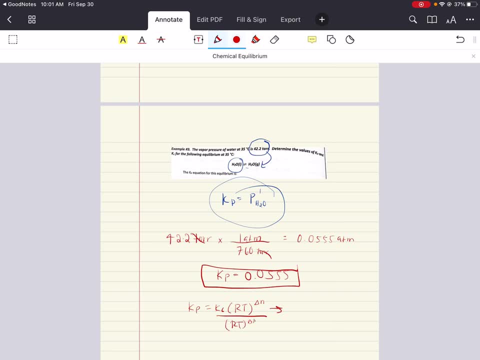 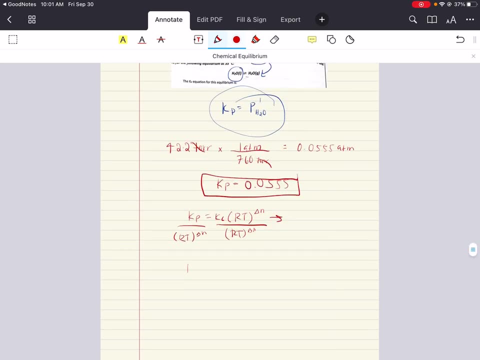 in order to do this is divide each side by r t delta n to the power of delta n. all right, in doing so, we get an expression for kc that is equal to rt to the power of delta that is equal to- i'm so sorry- k? p divided by r t delta n. now we have all these values except delta n. delta n is just um the.